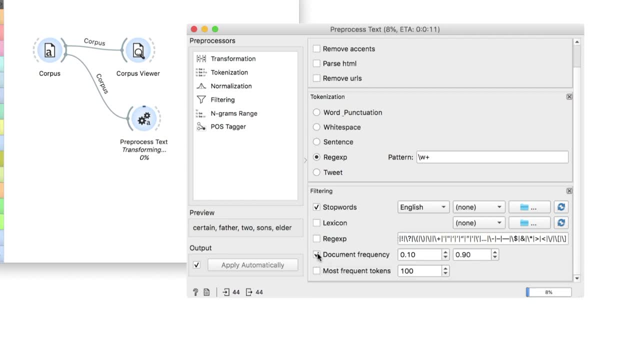 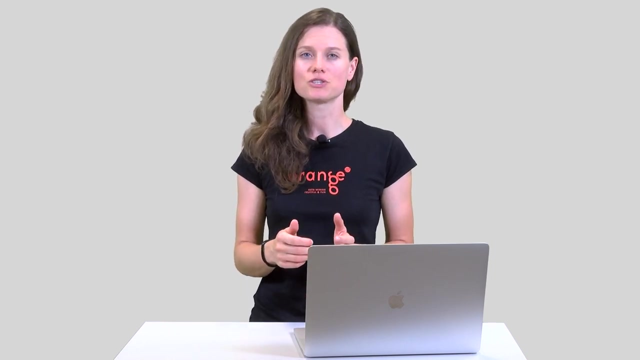 Finally, since we have long texts, we will remove words that appear in less than 10 percent and in more than 90 percent of the documents. Now we are ready for word embedding. Embeddings are a low-dimensional representation of high-dimensional data. They start with: 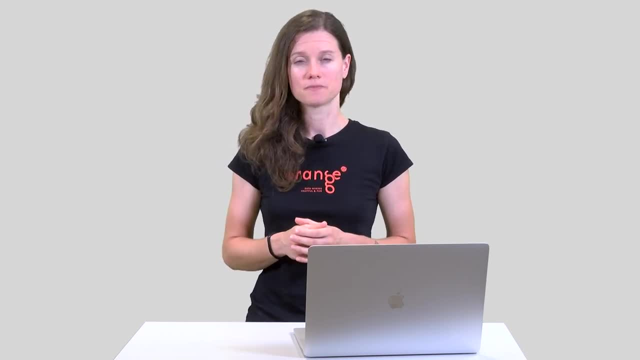 a single token, which, in our case, is a single word. They are based on two different types of data. They are the index and the index. In our case, these two are the index and the pre-trained models for the selected language, which looks at the word and places it in its 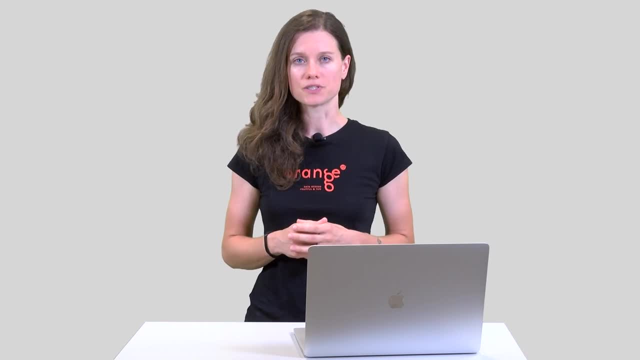 corresponding vector space. In other words, it embeds it. In this way, words that have similar meaning or come from the same family will be placed close together and will have a similar embedding vector. Once all the words are embedded, the procedure then averages. 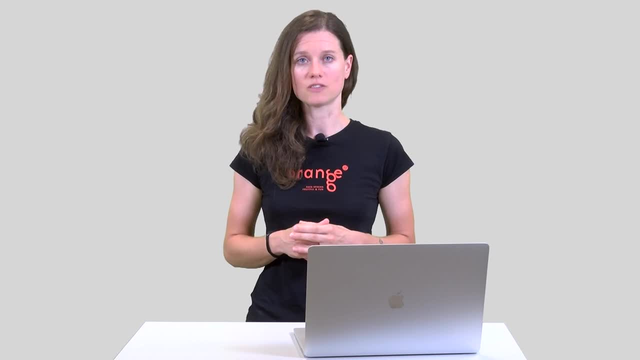 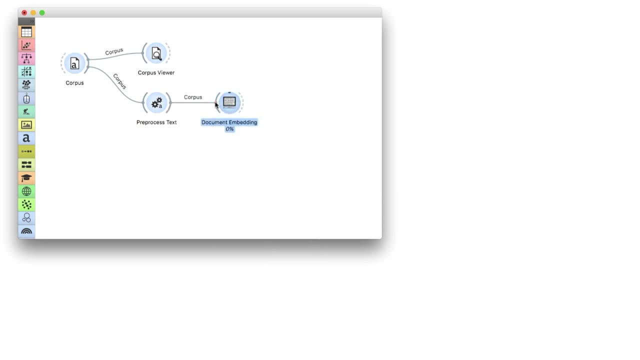 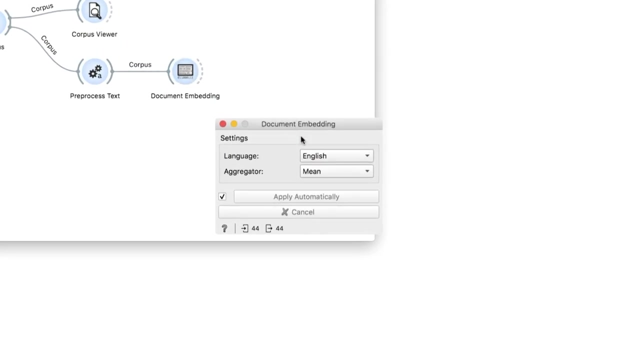 all the word vectors to produce a single document vector. In practice the procedure is simple: Connect document embedding to preprocessed text and Orange will compute the result. server-side You can change the language of the model or the aggregation of word vectors. A quick look at the data table shows us we now have 300. 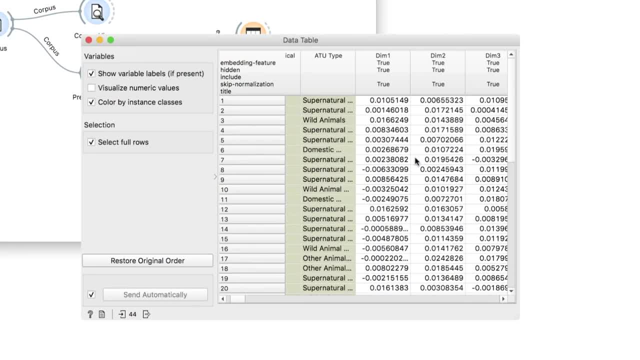 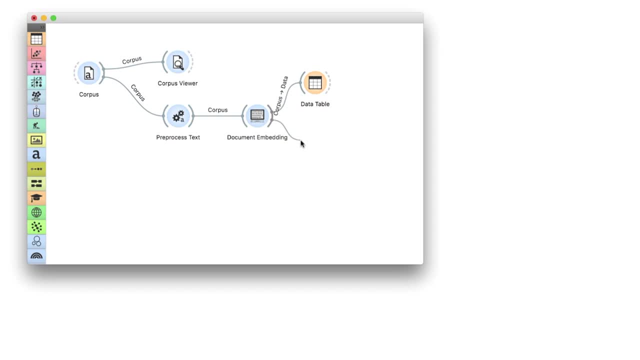 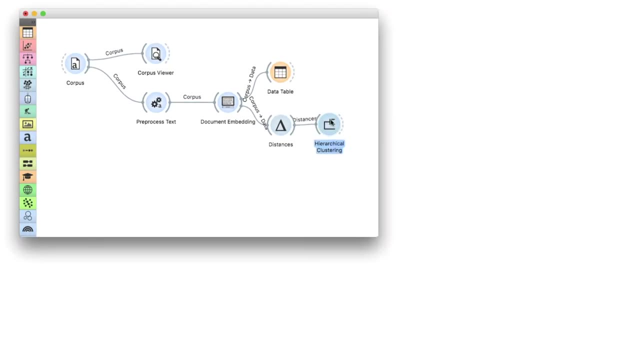 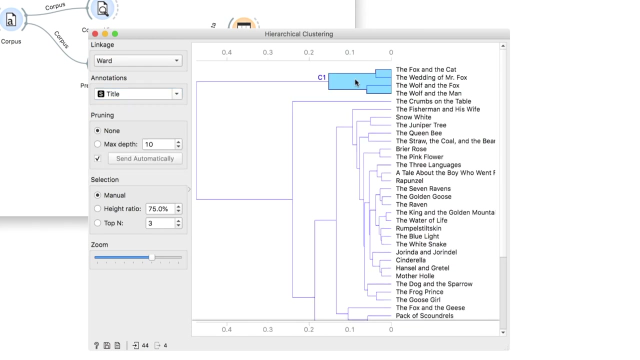 additional numeric features. Let us now do a simple clustering with cosine distances and hierarchical clustering with word linkage. I will label the tails by their title. A quick glimpse in the dendrogram shows us that animal-themed tails are clustered together based on the type of animal they 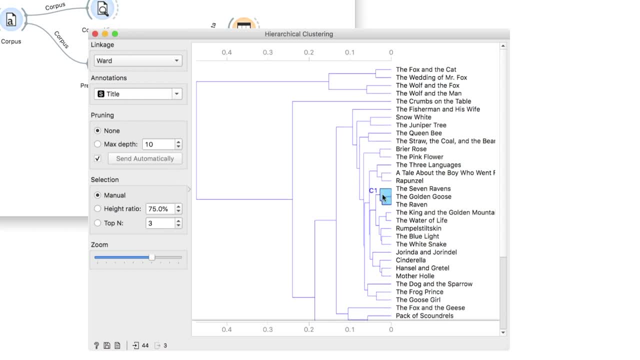 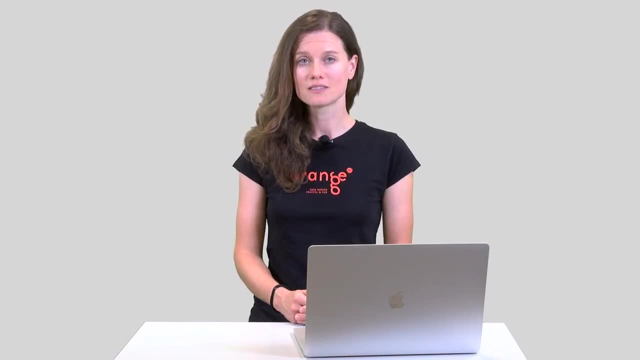 talk about. Document embedding is a great tool for describing documents with numbers. It is usually more accurate than bag of words, since synonyms are placed close together and, as such, the model doesn't rely on words alone, but also on their meaning. Bag of words, on the other. 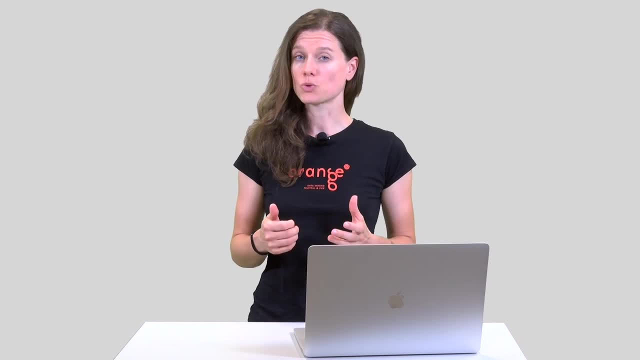 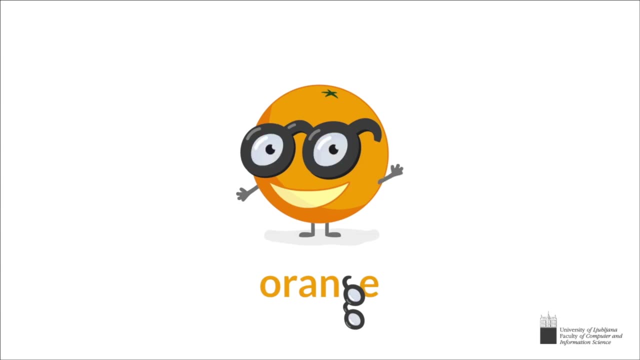 hand is easier to interpret. The choice of the technique is up to you. If you have any questions, please feel free to ask them in the comments.